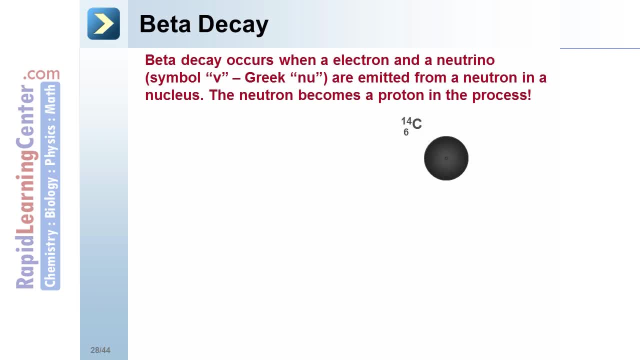 Beta decay occurs when an electron and a neutrino are emitted from a neutron inside a nucleus. In essence, the neutron becomes a proton. in the process, Beta decay results in a different nucleus or a daughter nucleus of the same atomic mass, but an atomic number which is one greater. 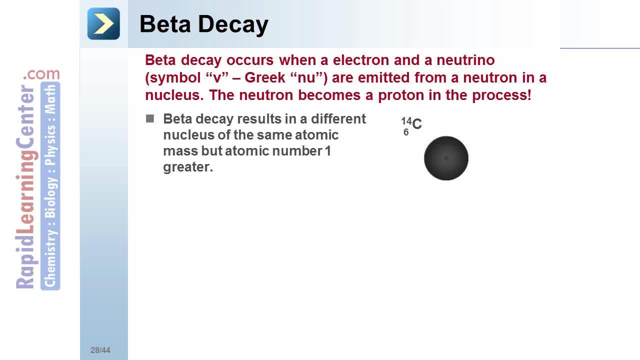 Thus, during beta decay, the element goes to a higher number on the periodic table, as you can see here. An example would be this: radioactive decay: Note: carbon-14 turns into nitrogen-14.. This is the result. This is the result. 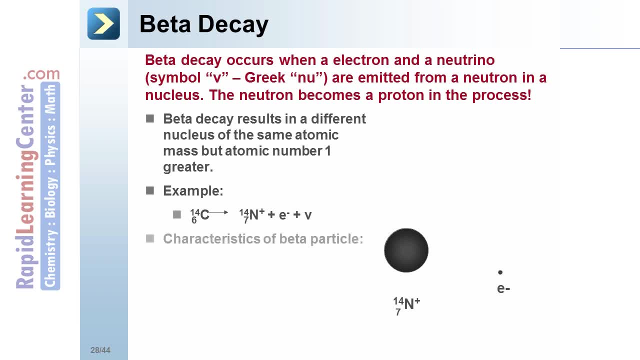 Plus an electron and a neutrino Characteristics of beta particles. They're small- They're an electron, after all- but faster and with more energy than an alpha particle. Thus they have a greater ability to penetrate materials than an alpha particle. 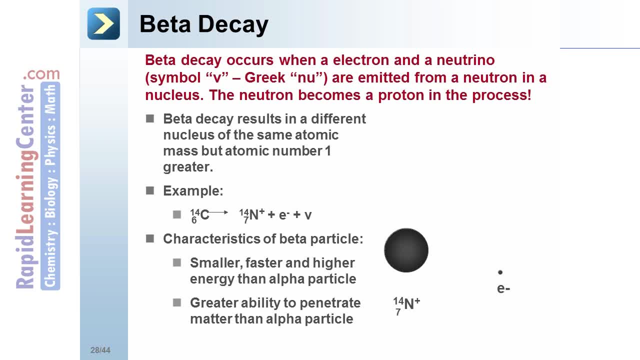 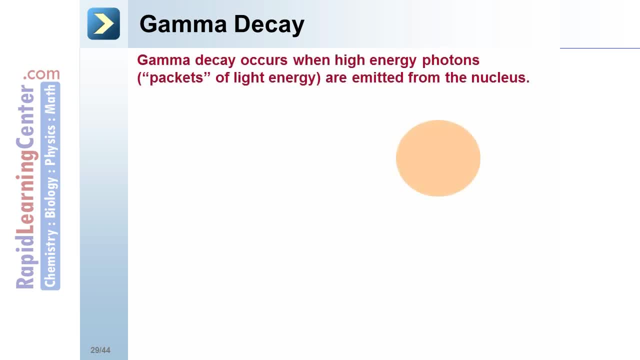 You would need thicker or more material to stop a beta particle- Gamma decay. Gamma decay occurs when highly energetic photons or packets of light are given off. Thus, gamma rays are very highly energetic. They have a high frequency of light. They are not matter at all. 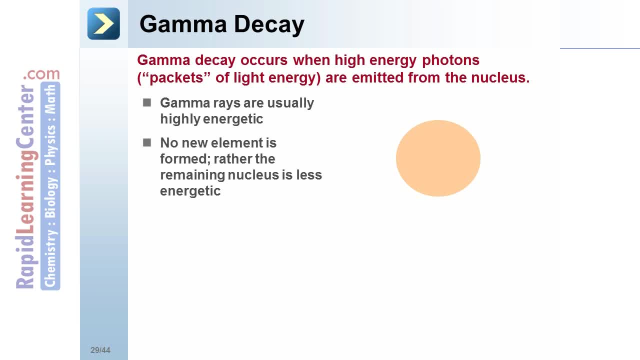 No new element is formed from this radioactive decay. Instead, the remaining nucleus is simply less energetic. It's now down to a more stable state: Ketogenicity, Ketogenicity, Ketogenicity. These particles are nervous, passive and gooey. 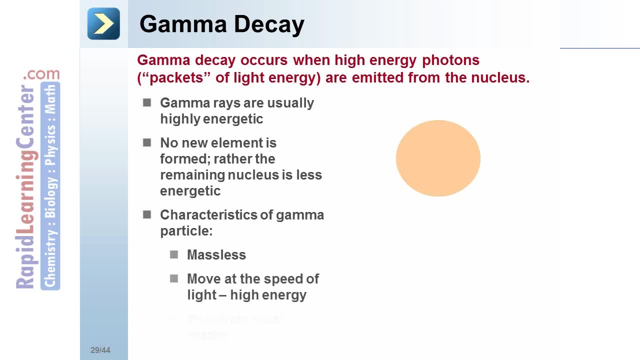 These particles have a say in being happy, Given that in some instances they may Hudson's, These particles may Hudson's 은 м Pokémon, M, Pokemon, Pokemon, Pokemon, Ultimatum Ultimatum. Exos stalk Ultimatum Ultimatum. Saturn Ultimatum. 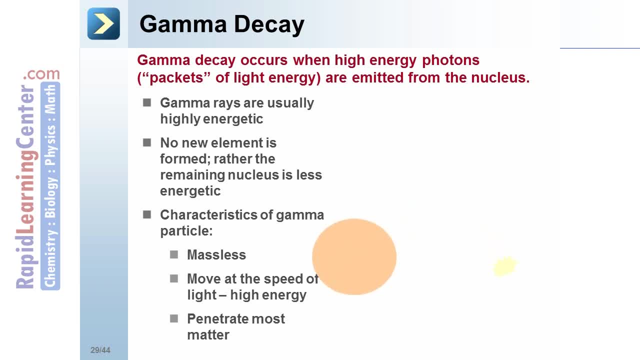 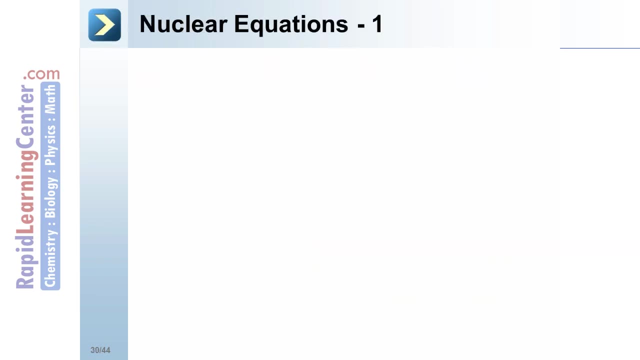 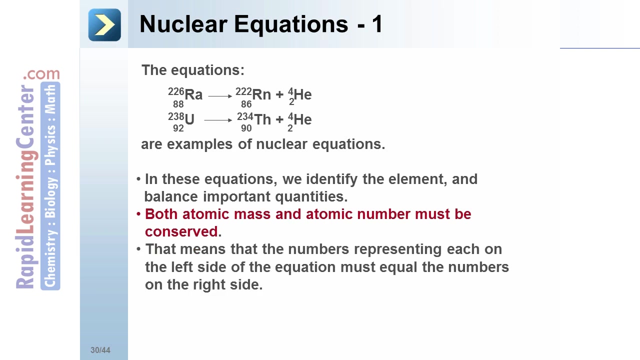 esy, a gamma ray, a photon of light, and becomes a more stable nucleus. Nuclear Equations. Here are examples of nuclear equations. Here we identified the element and can balance important quantities. Both atomic mass and atomic number, must be conserved. This means that the numbers representing each of those on the left side of the equation 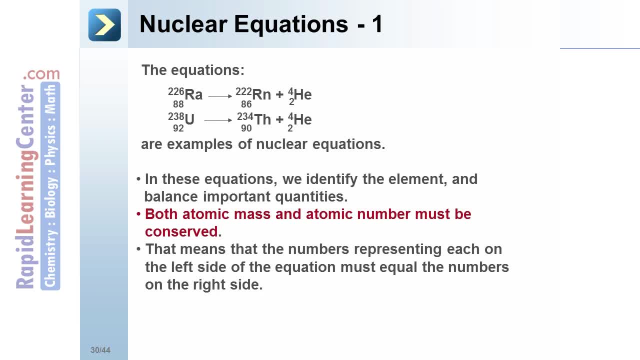 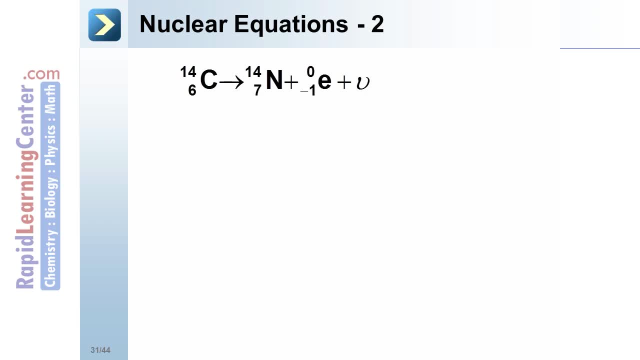 must equal the numbers on the right side of the equation. They must balance out Nuclear Equations 2. Take a look at this example. Here this equation shows an electron being emitted from a radioactive, carbon-14.. This forms nitrogen-14. 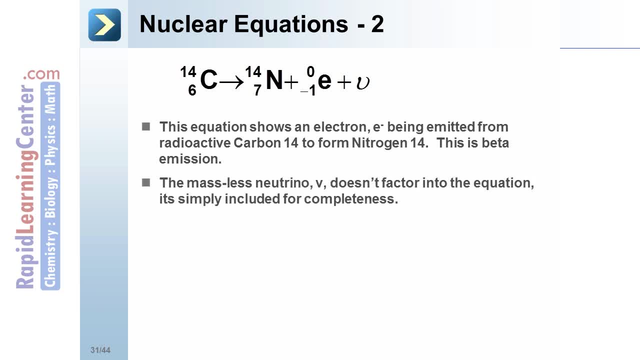 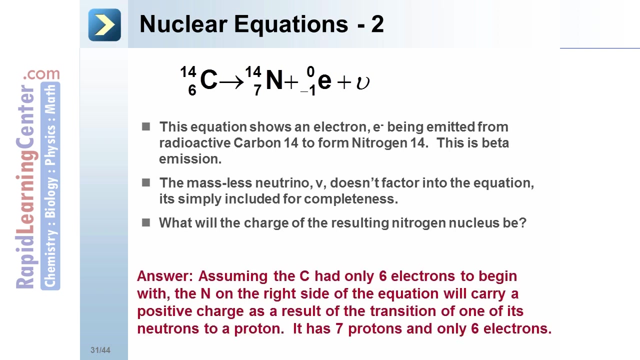 This is an example of beta radioactivity. The massless neutrino doesn't factor into the equation, It's simply included here for completeness. What will the charge of the resulting nitrogen nucleus be? Positive, Negative Or maybe neutral? Take a look at the equation carefully. 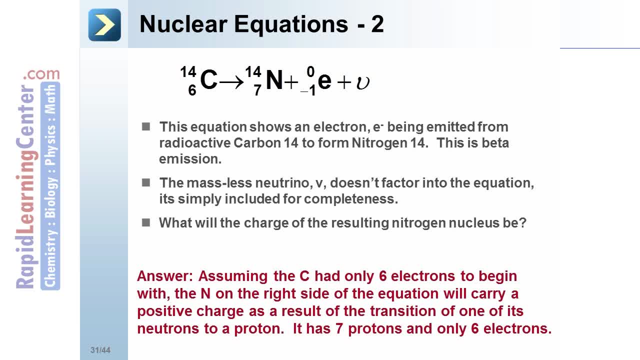 Assuming our carbon had the typical 6 electrons to begin with, the nitrogen on the right side of the equation must carry a positive charge. This is because the transition of one of its neutrons into a proton gives it 7 protons but only 6 electrons. 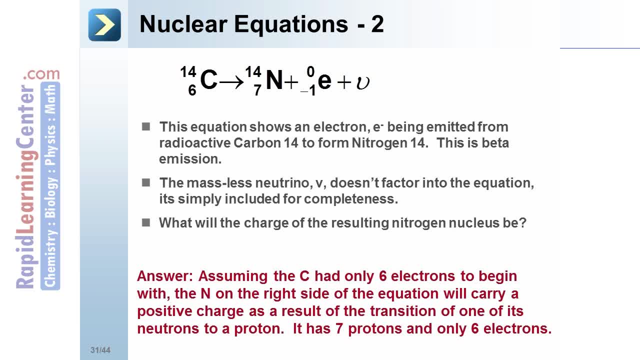 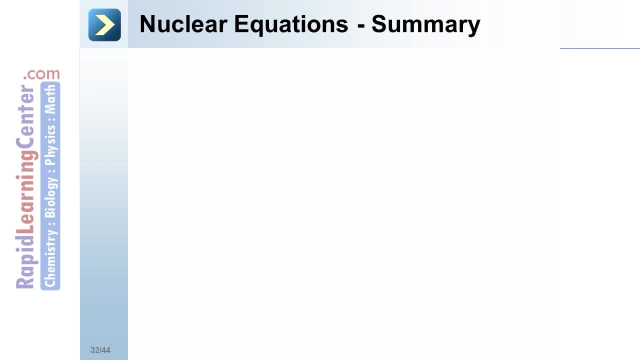 The ejected electron came from the nucleus. That is not part of the electrons from the typical electron. cloud 2 Nuclear Equations Summary. The Law of Conservation of Mass applies. This means the numbers representing the atomic mass on the left side of the equation must. 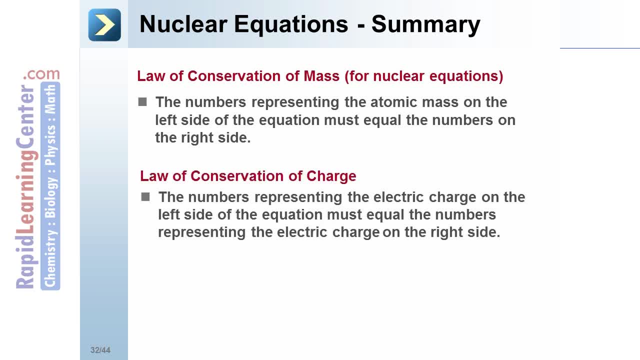 equal the numbers on the right side of the equation And the Law of Conservation of Charge applies. The numbers representing the electric charge on the left side of the equation must equal the numbers on the right side of the equation of the equation must equal the numbers representing the electric charge on the right side. 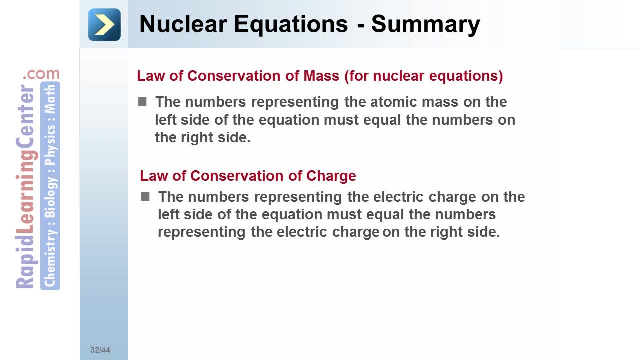 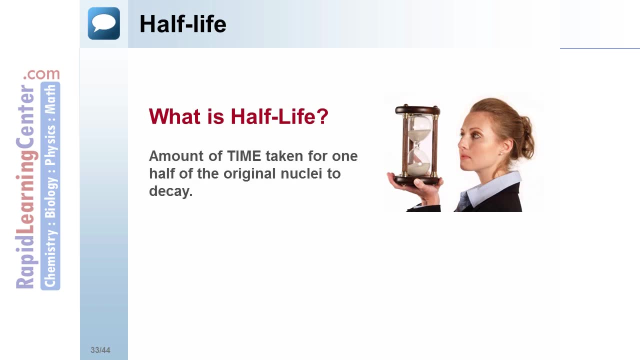 To simplify, the numbers on the top must add up and the numbers on the bottom must add up and be equal on both sides of the equal sign: Half-life. What is half-life? It's an amount of time taken for one half of the original nuclei to decay away into. 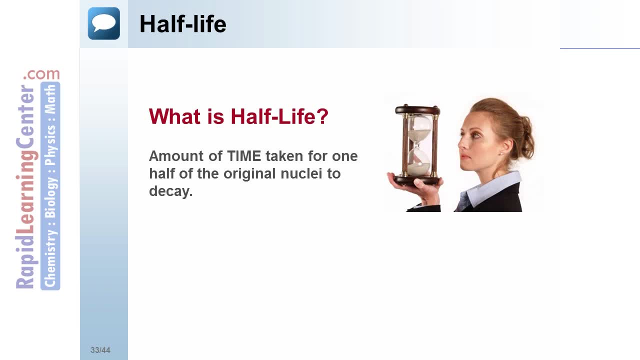 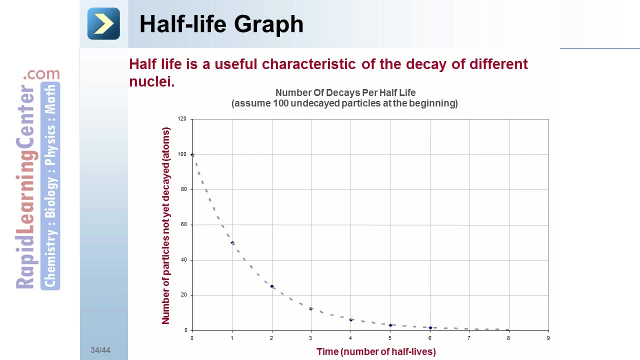 something else: Half-life graph. Half-life is a useful characteristic of the decay of different nuclei. Take a look at this graph, which shows time on the x-axis in number of half-lives and number of particles not yet decayed On the y-axis. 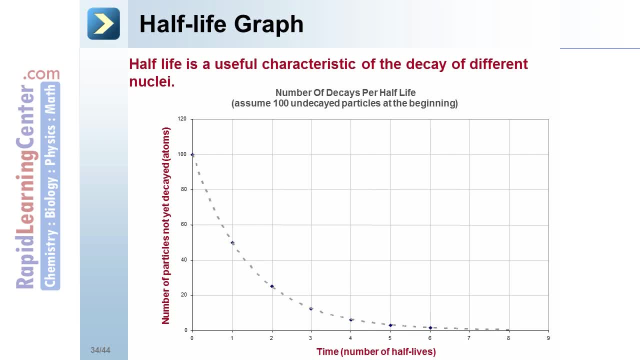 You can also think of this y-axis as a percentage Note. we start with 100%, then after one half-life we're down to 50%, then after two half-lives down to 25%, then three half-lives down to 12.5%, etc. 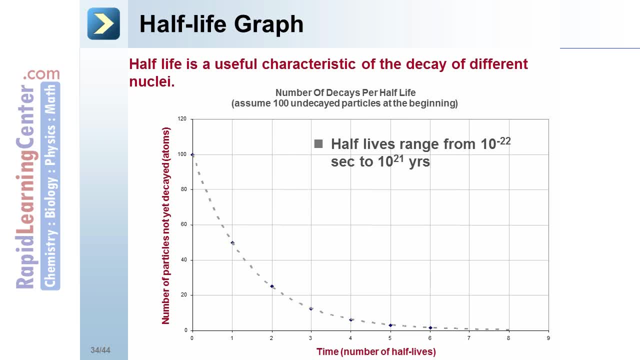 Notice that the graph is not linear. The half-lives of various elements can go from very, very short times to very, very long times, And these half-lives differ for each type of nucleus decaying, the type of element or isotope. 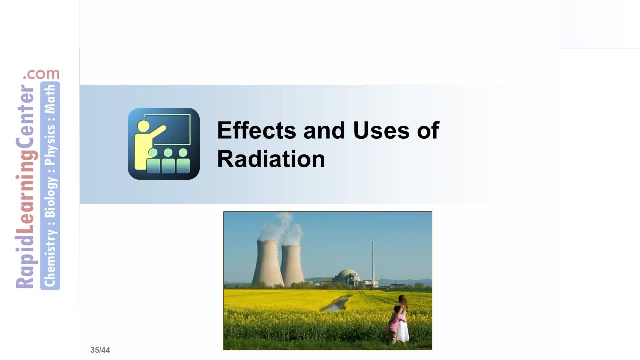 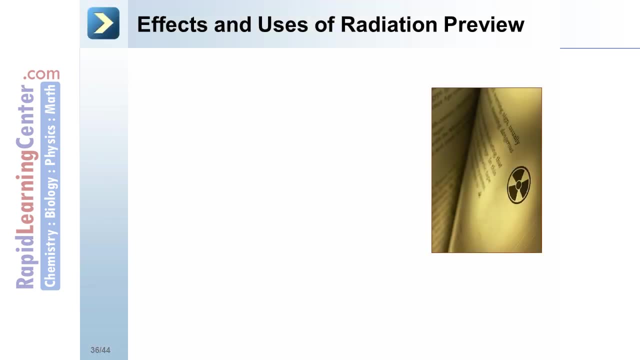 Effects and uses of radiation. Here we will describe some of the beneficial and harmful uses for radiation. Effects and uses of radiation. preview: Radiation is both useful and hazardous. It is both critical and helpful. Nuclear power plants have provided energy for half a century. 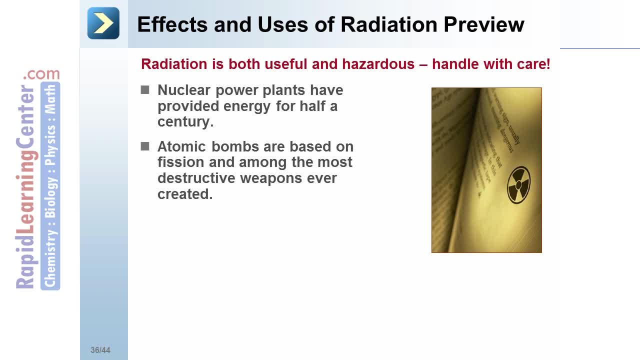 Atomic bombs are based on nuclear fission and are among the most destructive weapons ever created. There are many medical applications of radioactivity. Some examples are cancer therapy tracers, PET scans and MRIs Fission. This is the most common type of radiation. 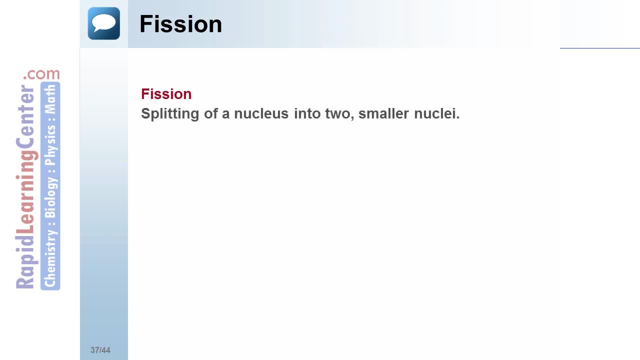 Fission is the splitting of a nucleus into two smaller nuclei. Here's an example equation showing fission. Note how we have one very large nuclei to begin with. then it is split into two roughly equal halves. Also note the neutron in the beginning and five neutrons afterwards. 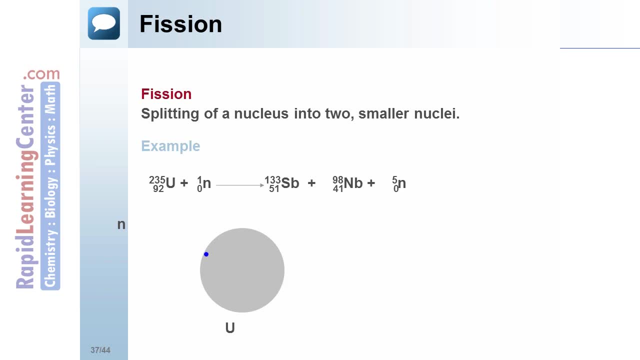 Here's our uranium nucleus, which absorbs a neutron, which then triggers the reaction, splits the nucleus and we have as a result, two smaller nuclei energy released and five neutrons Fusion. the opposite of fission Fusion is the combining of smaller nuclei or particles to make larger ones. 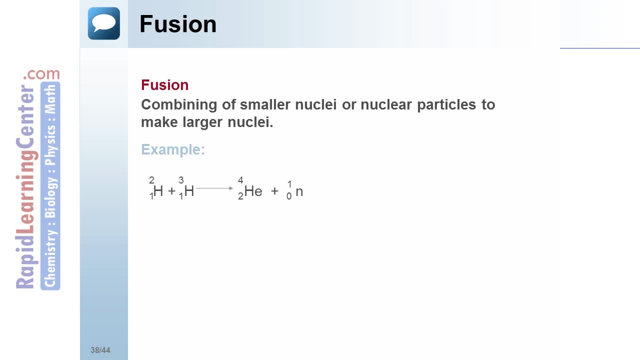 Here's an example equation. Note how we begin with hydrogen, but fuse it together to make a heavier helium nucleus. Here are our hydrogens, Here are our neutrons. They fuse together, producing a larger nucleus of helium, a neutron and once again a large. 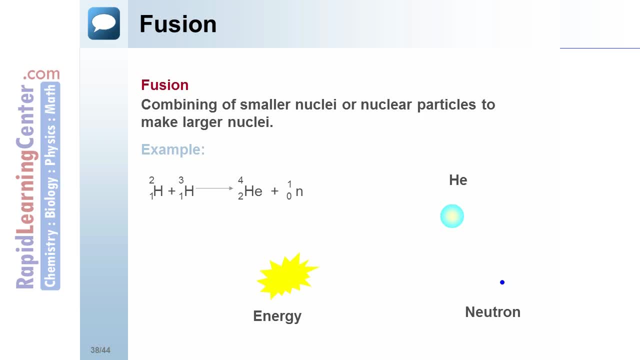 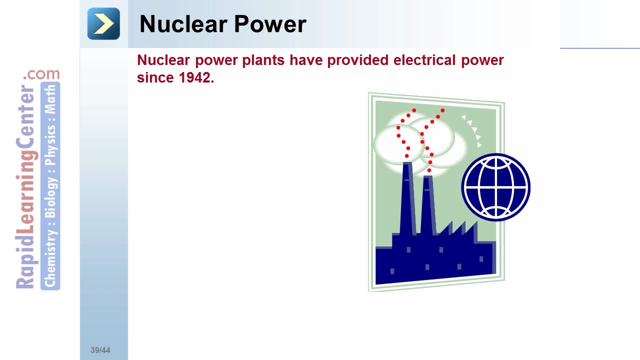 amount of energy is released. Here's another example equation: Nuclear power. Nuclear power plants have provided electrical power since 1942.. Fission is the reaction that gives rise to a continuous chain reaction that is self-sustaining. This self-sustaining reaction is known as fission. 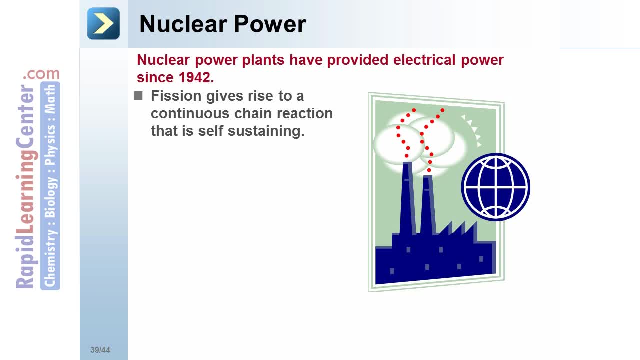 This self-sustaining occurs because of those neutrons that are released during the fission reaction. They go on to fission other atoms. The reactions are slowed or controlled by control rods or moderators, And nuclear power presents different risks than typical forms of power generation. that is compared to 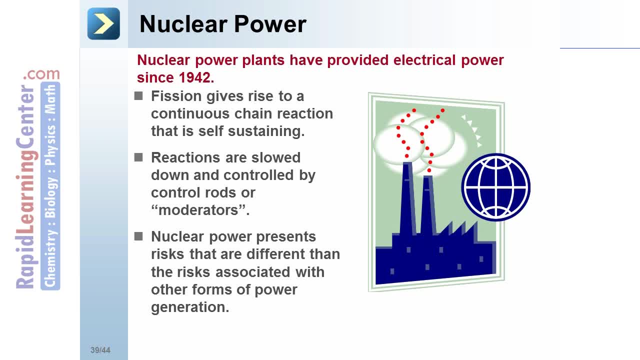 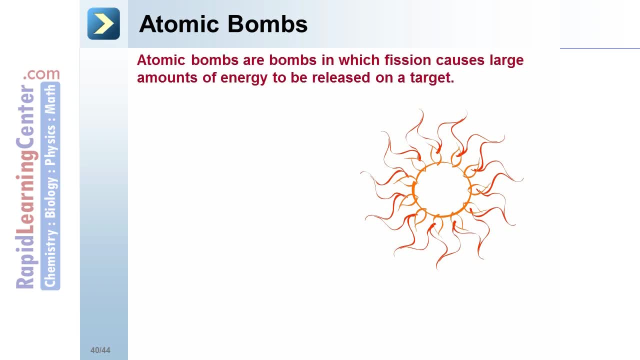 burning fossil fuels. It also provides some advantages, too. Atomic bombs: Atomic bombs are bombs in which fission causes a large amount of energy to be released on a target. These were first built in the early 1940s and dropped on the